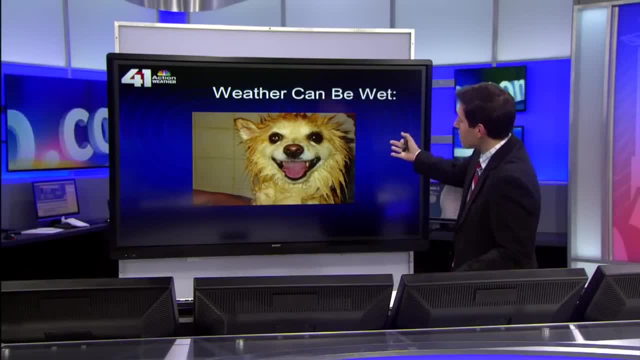 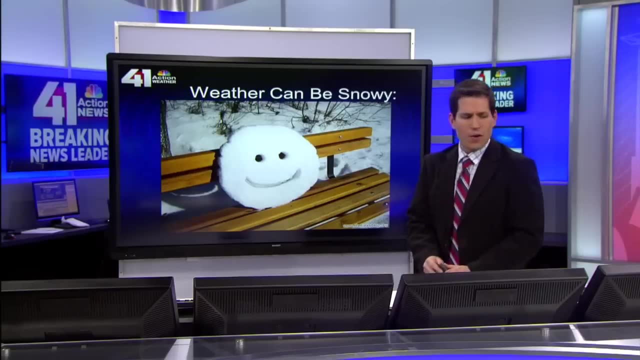 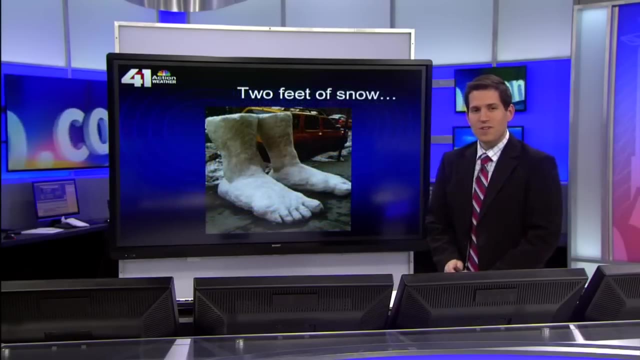 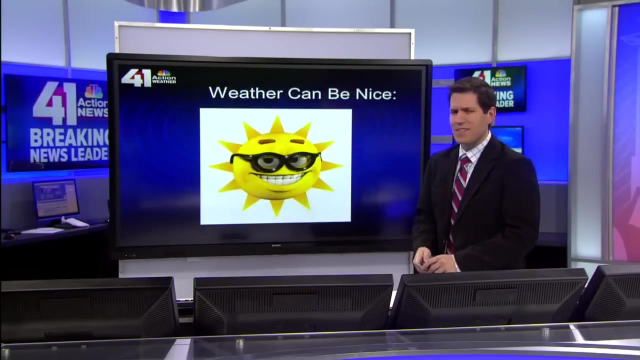 can be several different things, kind of like this doggy right, The weather can be wet. What a cute little pup. What else can the weather be? It can be snowy, and hopefully you're happy when there's snow out there. Have you ever seen two feet of snow before? Do you want me to show you two feet of snow? Look, there's two feet of snow, See. you don't see that around here very much, do you? No, not at all. What else can the weather be? It can be sunny and nice. That's a pretty bright and happy sun. He's bright because he's got sunglasses on and regular glasses. He's 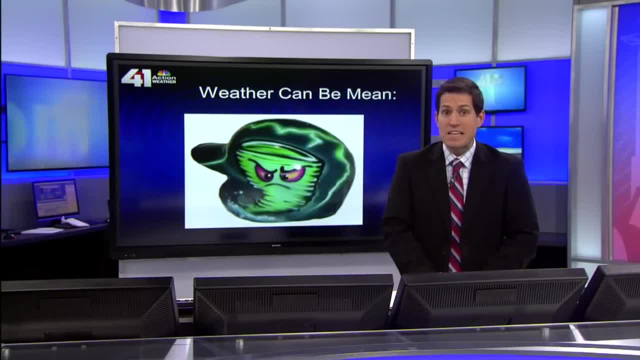 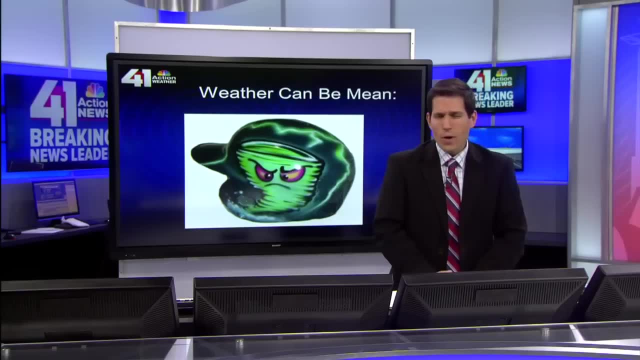 smart. He's a smart son. You know what else the weather can be. It can be mean, Yeah, like during tornado season, right, Any of you see any big scary storms? Yeah, they're kind of scary and mean We. 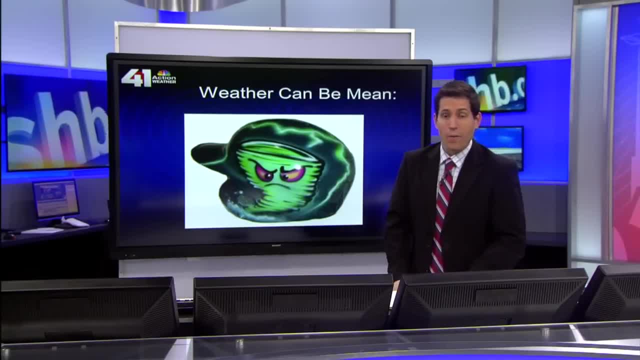 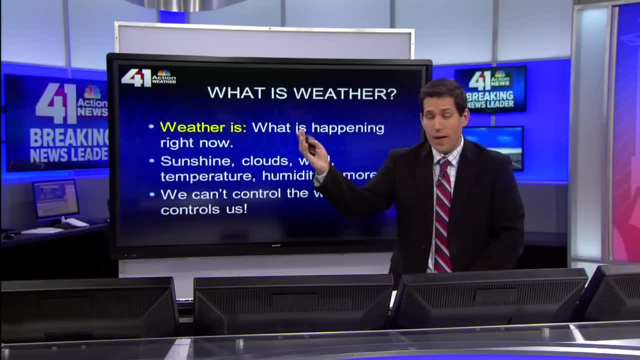 don't like scary storms, so hopefully we can keep those away for a while. So let me ask you a question: Do you know what weather is? Weather is what's happening right now. If you can look out the window, go outside. you know what's happening. That's the weather. If it's sunny, if it's warm, 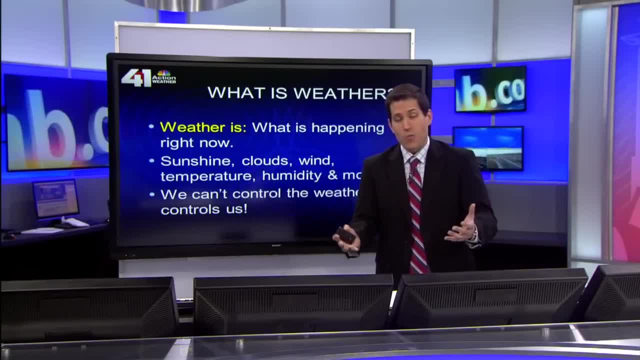 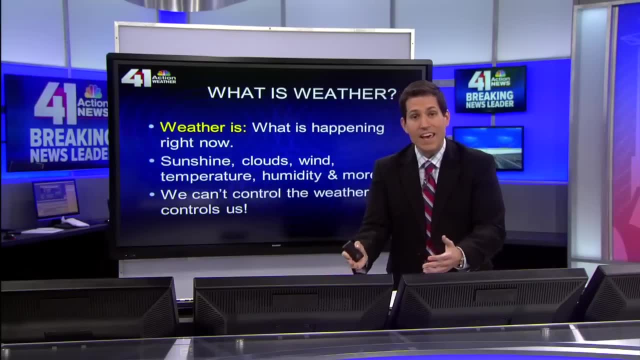 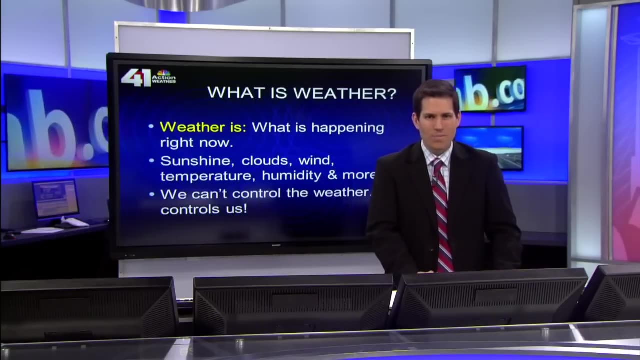 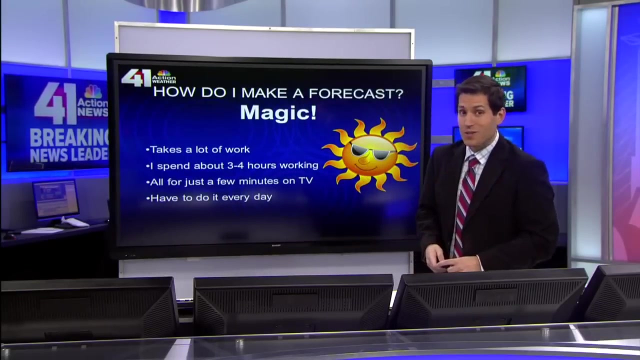 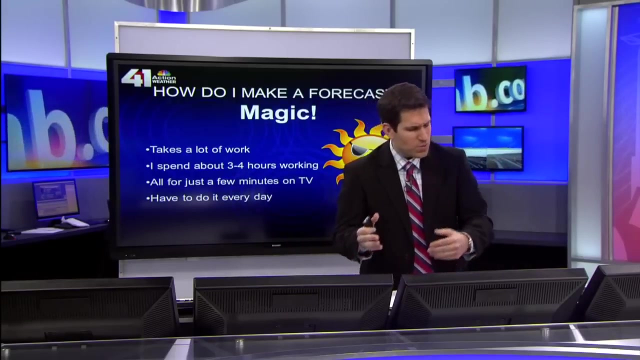 if it's cold, if it's raining, if it's storming. that's all the weather. And the really neat thing about the weather: we can't control it. It controls us. If you wore shorts today, if you wore a coat today, that's because the weather made you do it. You didn't choose it. You had to because of the weather. I want to talk to you about a couple of things that I do my job. What is it that I do as a meteorologist on TV? Well, magic. There's a little bit of magic in what I do. It takes a lot of work. I spend a few hours each day working and looking over all kinds of papers and forecast stuff. Do you want to do? you want to see some of what I do? 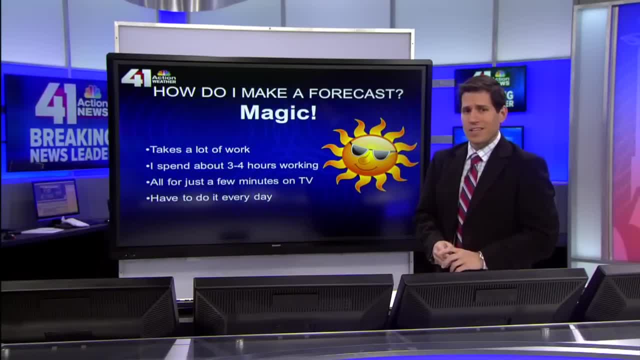 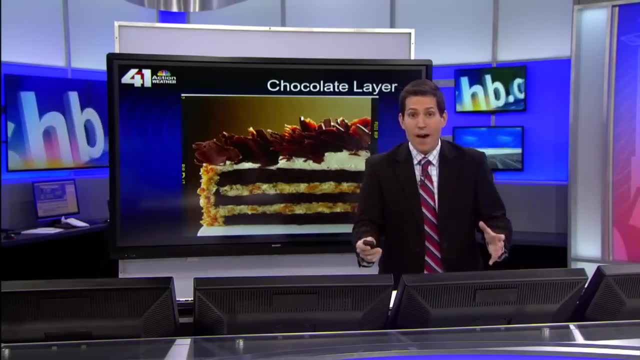 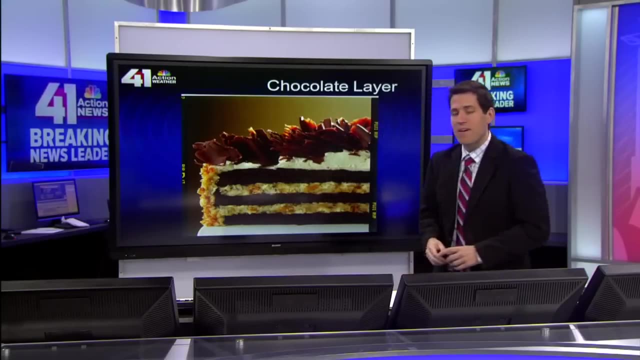 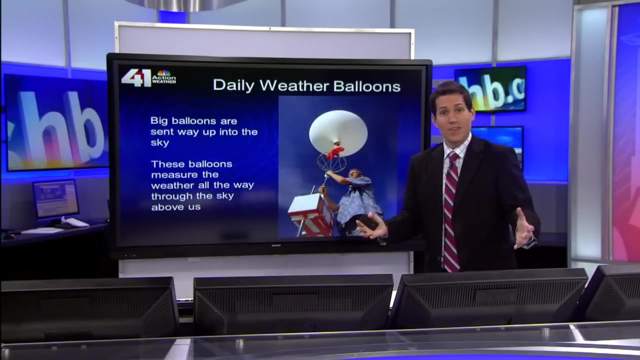 Okay, here's an example of what I do. Do you like cake? I love cake. Think of cake. Look at all the layers in that cake. right, That's kind of how the atmosphere works, The earth, the air around us, And that's what I study is all the layers that we have in the atmosphere And that's how we predict the weather. How do we do that exactly? Well, let me show you. You like balloons. We take these big, giant balloons and we send them way up in the sky. 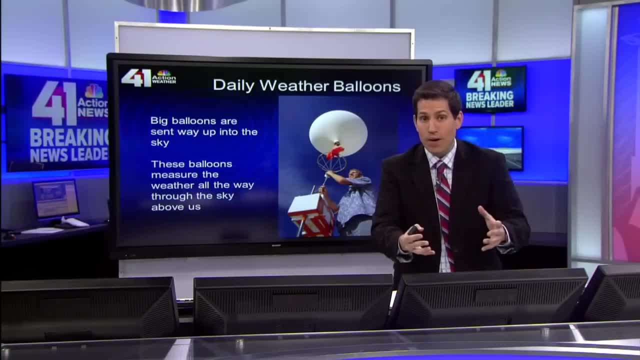 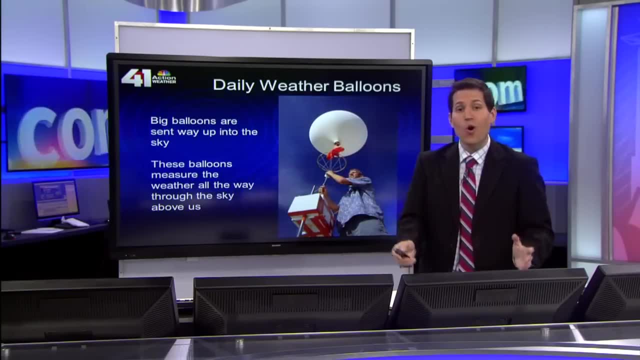 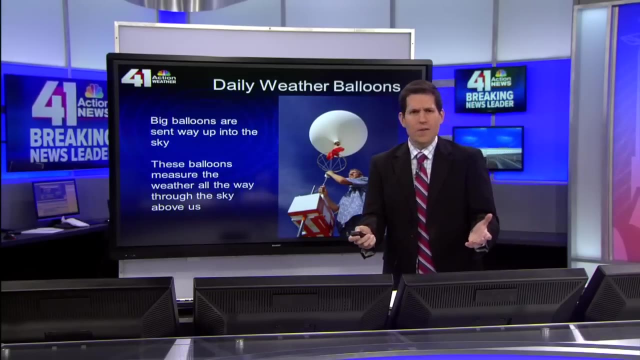 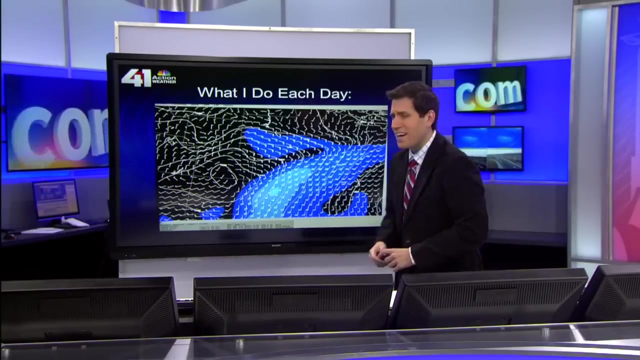 And when we do that, we measure the temperature and the air pressure and other things in the atmosphere. That way we can know what the weather is going to do. And we have all kinds of balloons all over the country to help measure the weather, high up above us, way up in the sky. Well, what do we do with all that information? Well, it comes back into a computer and then I do things like this. I look at these charts with all these colors and these lines on there. It's really geeky, It's kind of nerdy. Look charts like this that tell me where it might rain. 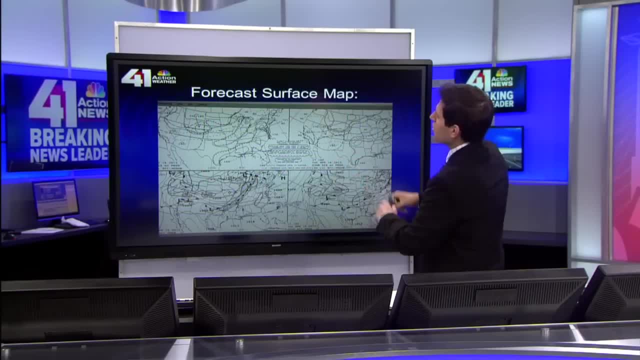 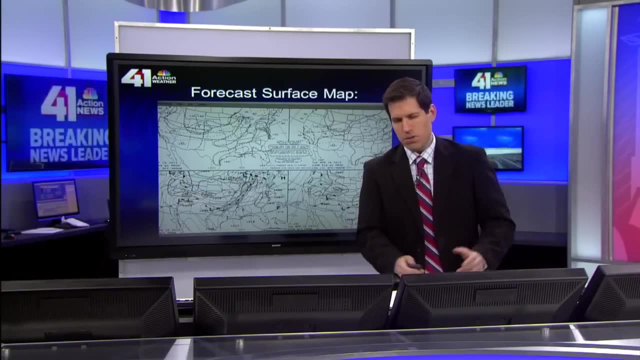 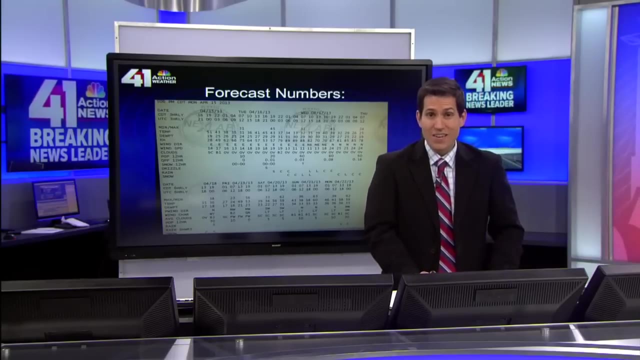 Charts where it shows me there's a warm front, Even big, scary charts like this. Lots of drawing: I do lots of drawing and coloring in my job. sometimes I try to stay within the lines, but not always. What else do I do? I look at a lot of numbers, a lot of math and science, And if you like math or science, if you do, maybe you could be a meteorologist someday. There's a lot of numbers that I have to work with. Also, we use things like radar and satellite. You've seen me talk about this on TV before right, When the clouds are in. 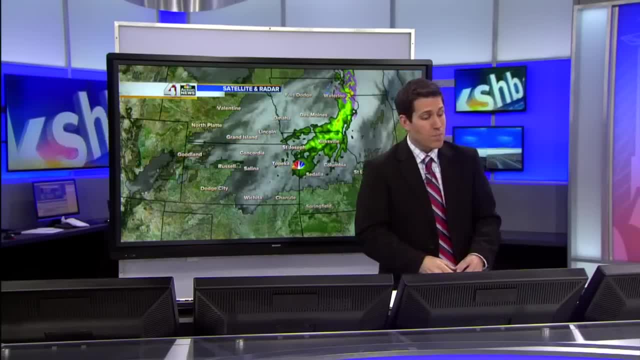 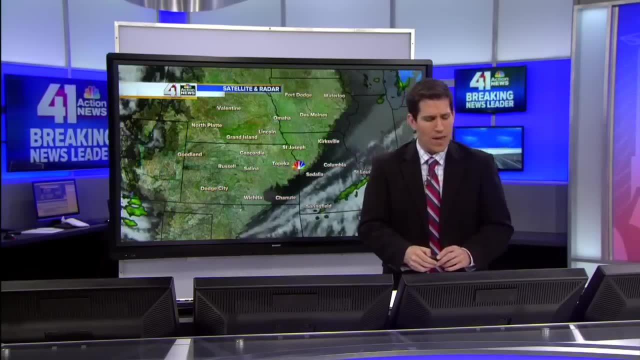 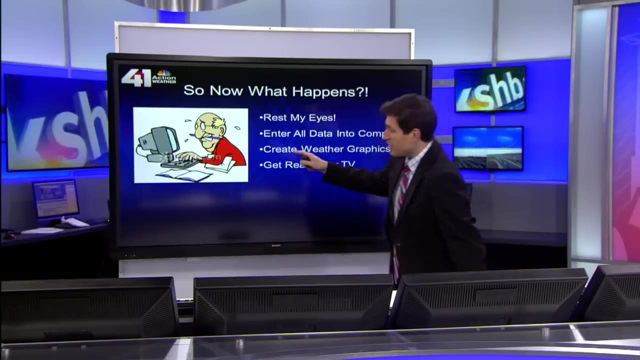 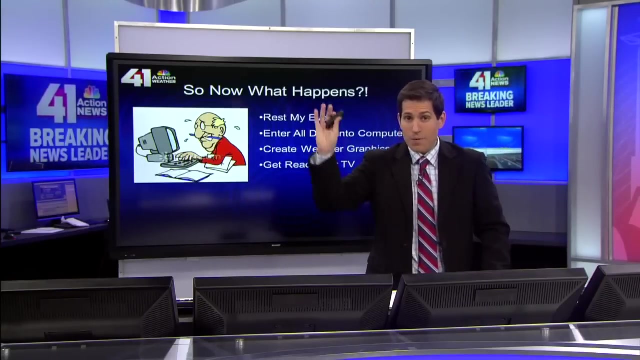 that's on the satellite. The radar shows the rain, shows us when it might storm, and things like that too. That's one of the ways that we do this is with radar and satellite, one of the many tools that we have. So what happens after I look at all these things, all those layers in my cake? What do I do? Well, I put it all together. Then I sweat and I work at the computer and I type in everything that I can to get ready for the news. Have any of you seen me on the news before? Does your mom or dad watch the news? Can I tell you something? There's magic. 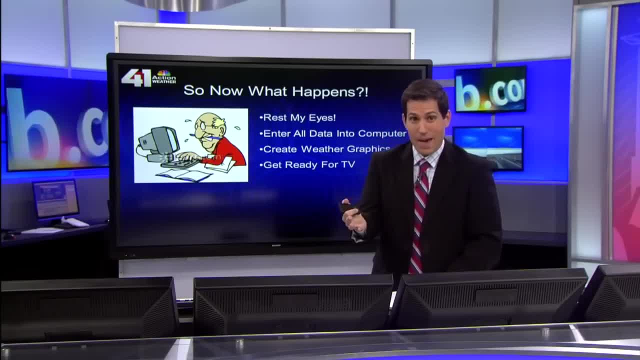 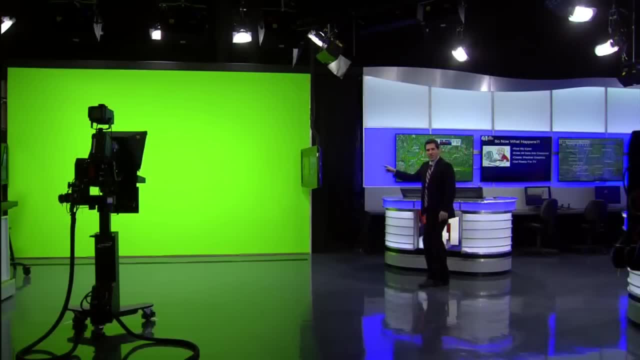 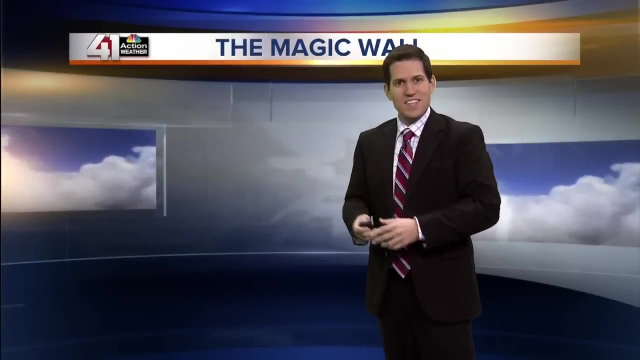 There's magic in this room. Do you want to see some of the magic? This is the boring stuff. Let's go take a look at some of the magic. Let me show you some magic that I have. Look at this over here. This is my magic wall. This big green wall is where I stand. You don't usually see this on TV. We can't show it to you, But let me show you some magic of what happens when I step in front of this wall. Does this kind of look familiar? now, Hang on, Let me go back. Let me go back real quick. See, there's no magic.